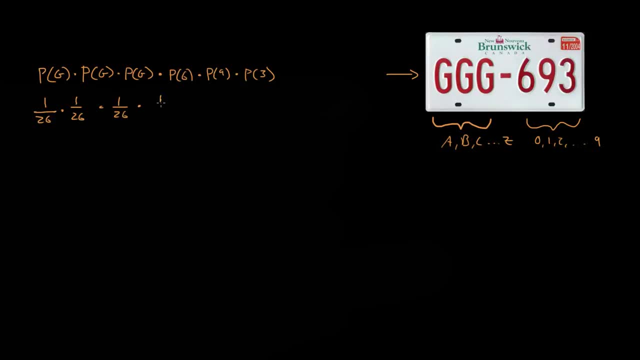 And now, what's the probability of getting a 6?? Well, that's one number out of a total of 10.. 10. So we have 0 through 9.. So there are 10 digits. So there's, there's. we want this one digit out of a possible 10 digits. 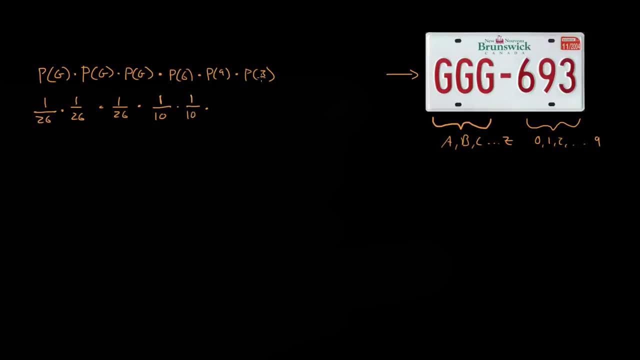 And then we do the same for the 9. So that's out of 10.. And the same for the last one, That's out of 10 as well. Well, now, there's actually a much simpler way of doing this. This is one. this is one thing that we want out of all the possible different types of plates. 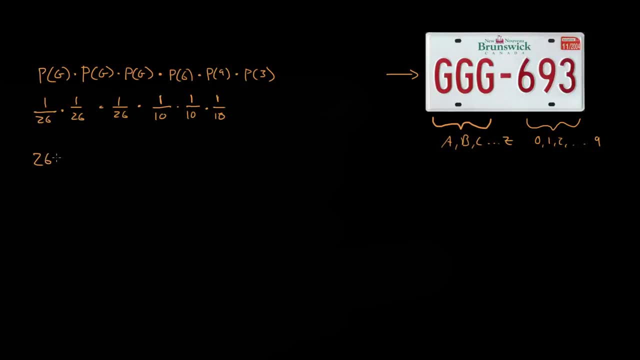 So we have an actual. we have actually 26 times. 26 times 26 times 10 times 10 times 10 will give us the total number of plates possible. So if we did a little bit of math we could find it out. 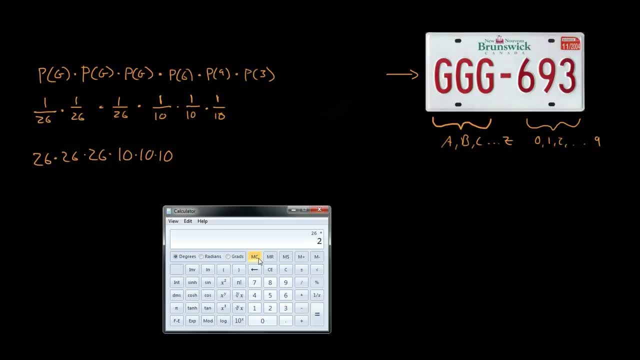 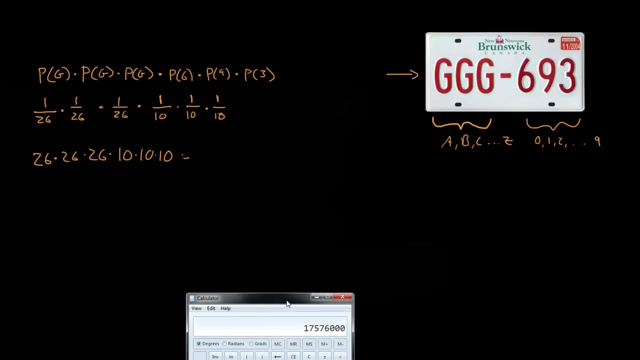 out the total number of plates possible. so that's 26 times 26 times 26 times 10. 10 times 10, that is equal to: that's a really big number, that is equal to whoops, see a thousand seventeen point five million, seventeen point five million. so 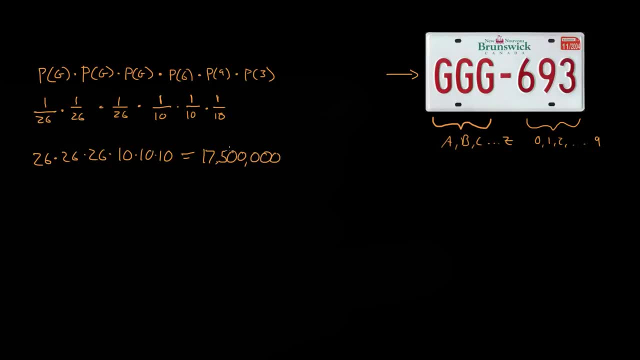 put a bunch of zeros. so really the probability of getting this one plate is one is one out of the seventeen point five million million. so it is really unlikely to get this plate out of anyone. let's see what we got here. let's see what we got here. let's see what we got here. 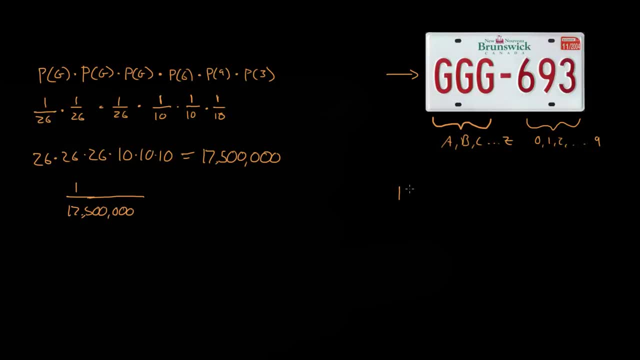 let's find the probability of getting one. so let's say we want a license plate. that was, that was a, b, c, 1, 2, 3. what's the probability that? well, getting an a is 1 out of 26, getting a B is 1 out of 26. and getting a C is 1 out of 26. and getting a. 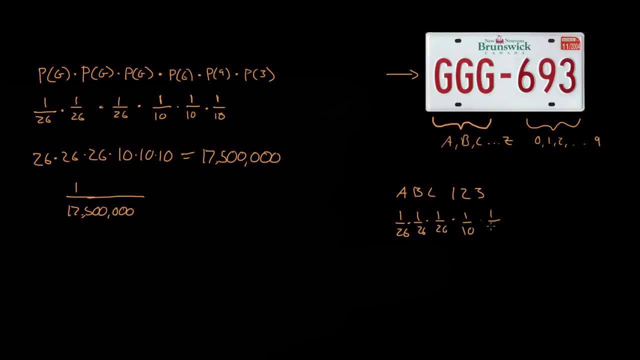 1 is 1 out of 10, getting a 2 is 1 out of 10 and getting a 3 is 1 out of is 1 out of 10- 10. so this probability is again 1 out of the 17 mil a million, 17.5 million. so